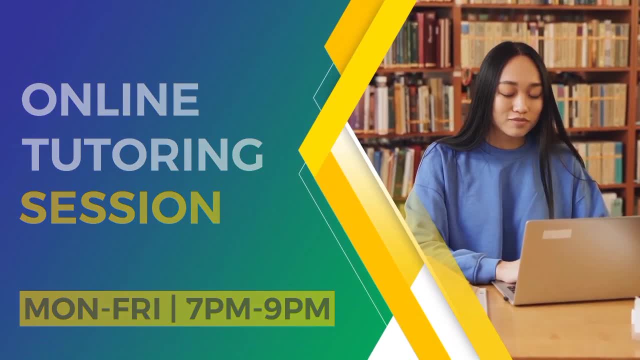 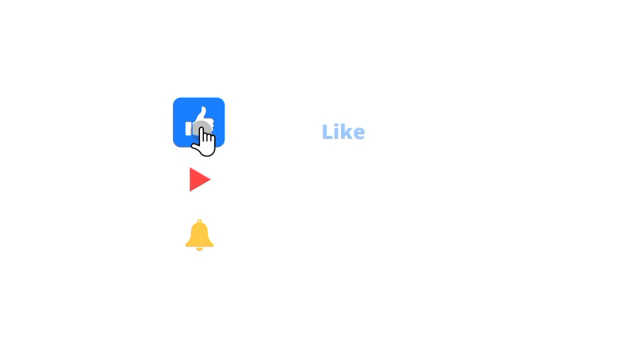 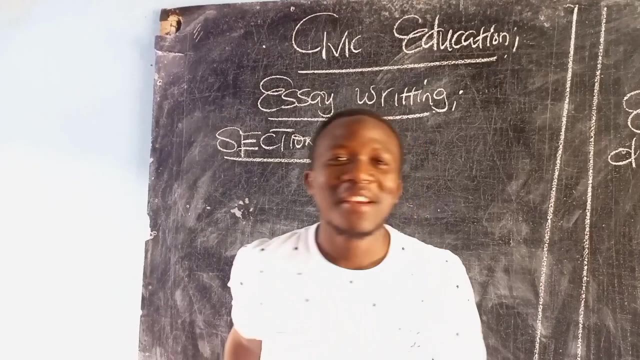 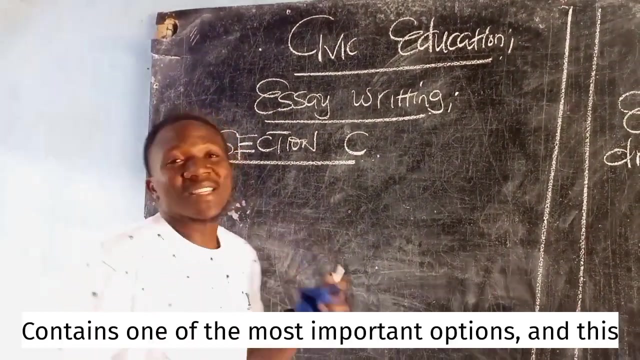 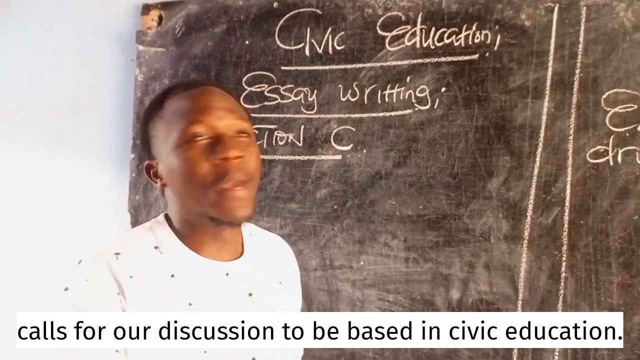 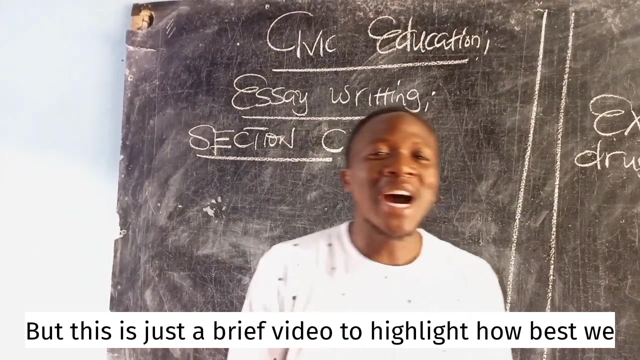 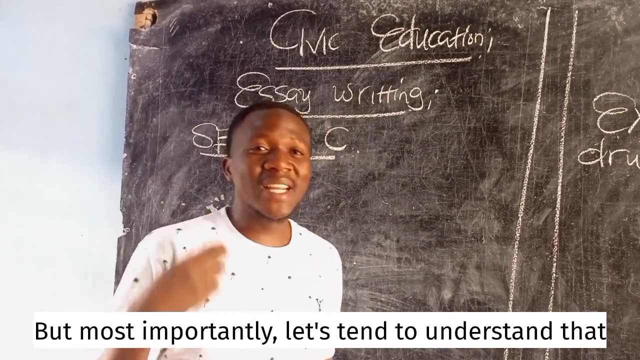 The following video in today's discussion contains one of the most important options, and this calls for our discussion to be based in civic education. But this is just a brief video to highlight how best we can handle Section C of nowadays civic education. But, most importantly, let's tend to understand that Section C is everything about essay writing. 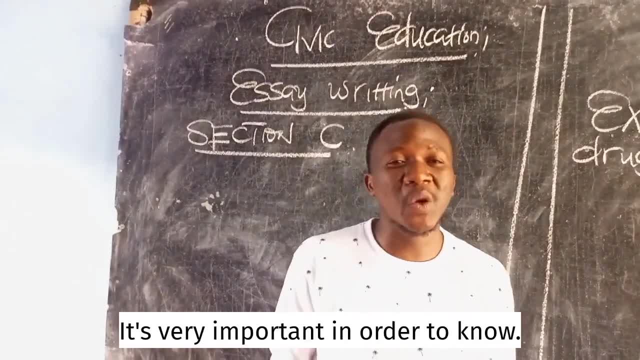 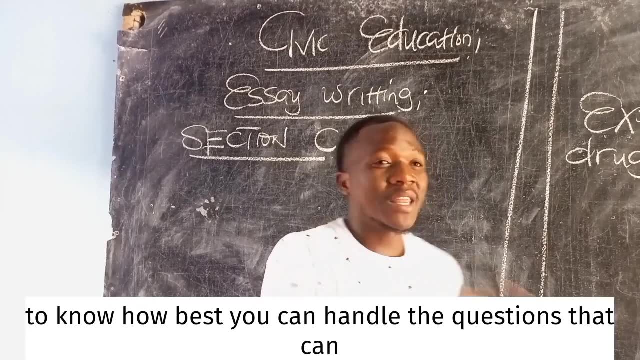 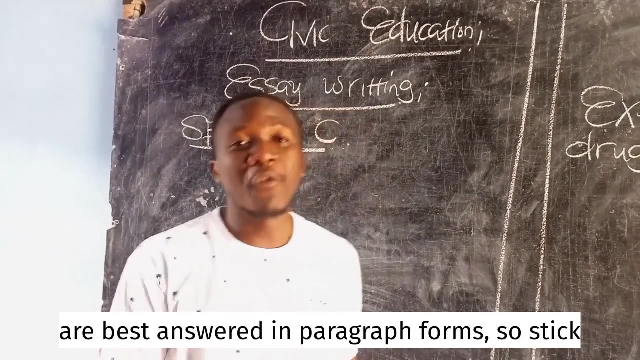 In an exam. it's very important in order to know Section A, Section B, and also it's very, very important to know how best we can handle the questions that can be able to be brought in Section C, as these questions are best answered in paragraph forms. So stick. 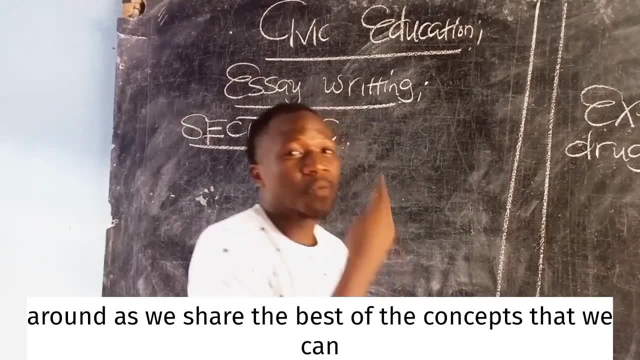 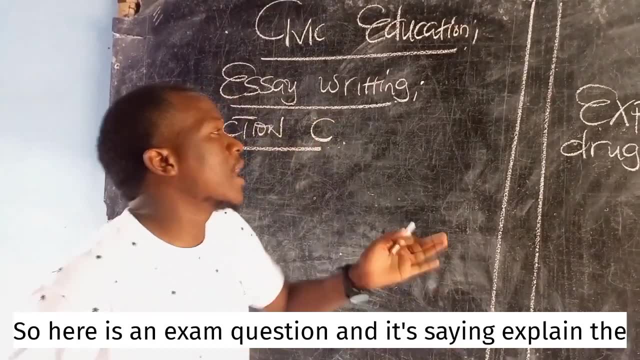 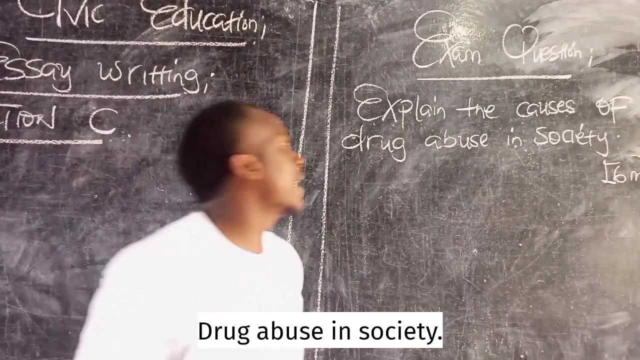 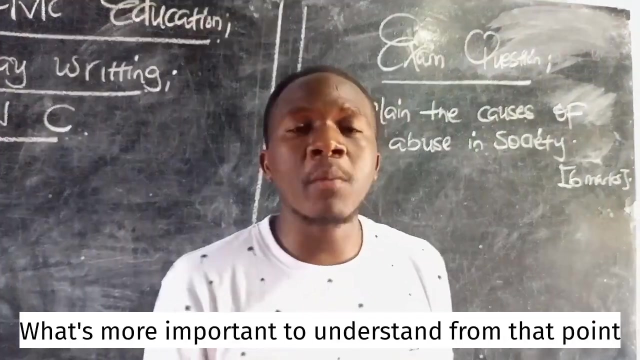 around as we share the best of the concepts that we can be able to utilize as we prepare adequately for the final exam. So here is an exam question and it says: explain the causes of drug abuse in society. What's more important to understand from that point of view is to relate to the number. 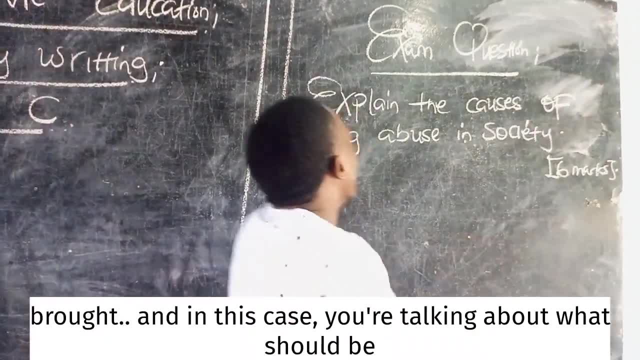 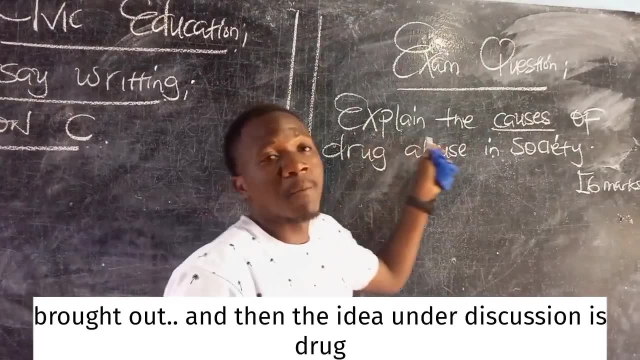 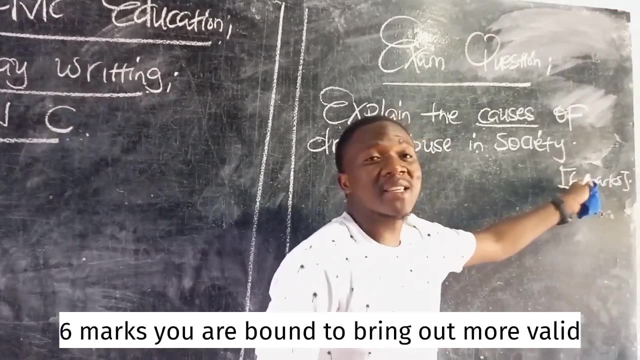 of marks that are brought, And in this case we are talking about what should cause. and then the idea of the discussion is drug abuse and its impact in society. How best is it brought about? When there are six marks, you are bound to bring in the most important one, and that's. 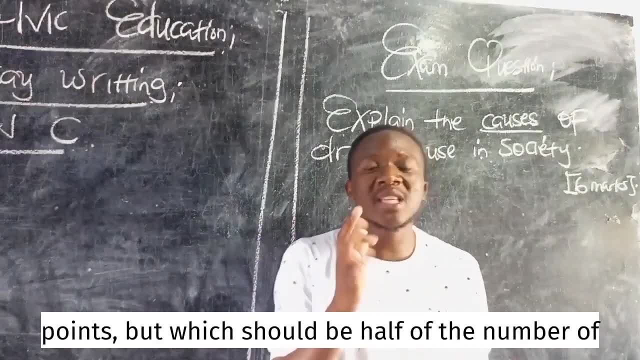 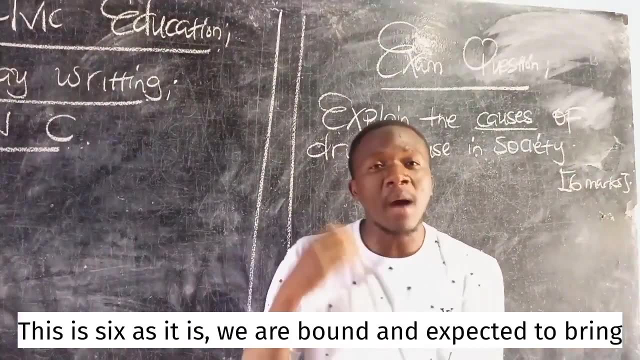 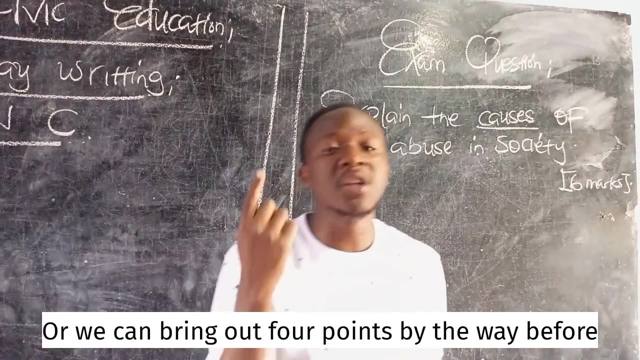 the first one. The second one is to bring out more valid points, but which should be half of the number of marks Provided. this is six. as it is, we are bound and expected to bring out at least three points, meaning we can bring out three or we can bring out four points. 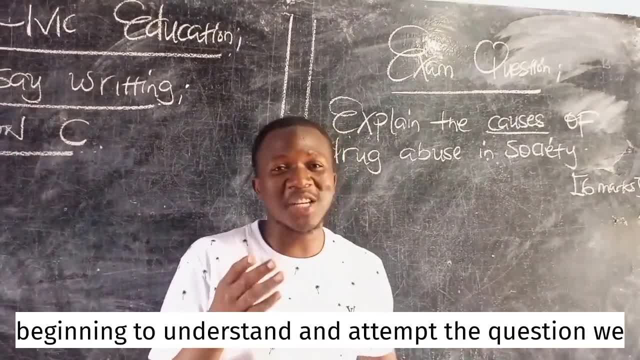 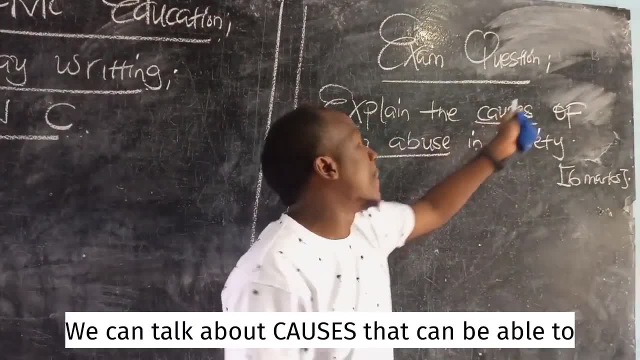 By the way, before beginning to understand and attempt the question, we are going firstly to just discuss a bit about drug abuse. Then we can talk about causes of drug abuse in society. I do think that this is the first step because, as you think about drug abuse and its impact, 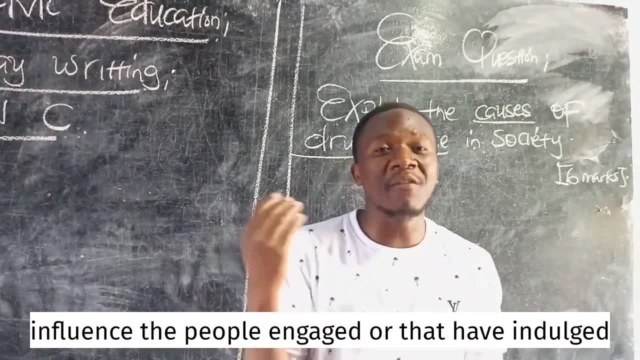 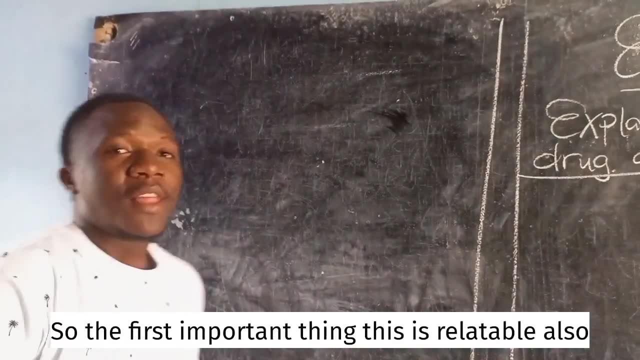 it also reminds you of psychosis, We are being told. these are things that can be able to influence the people engaged or that are endowed in it. So let's see what we have to do. So the first important thing: This is relatable also to biological pepora, as when you are 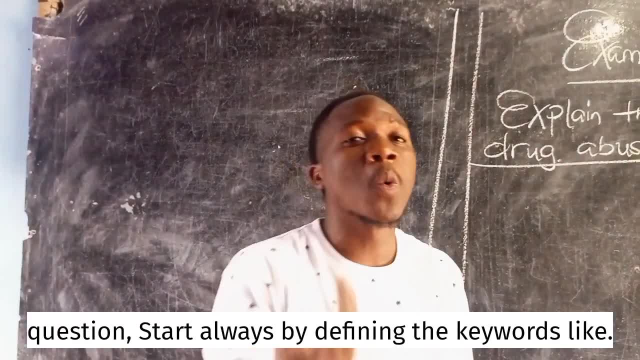 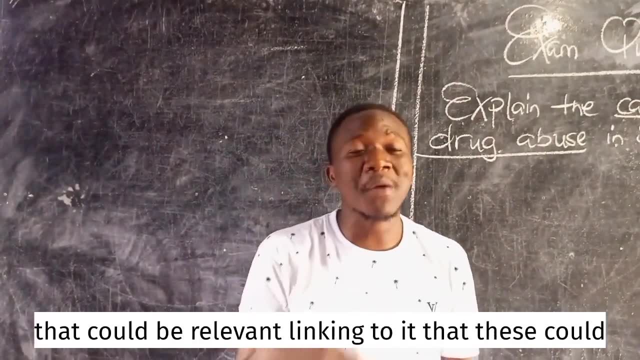 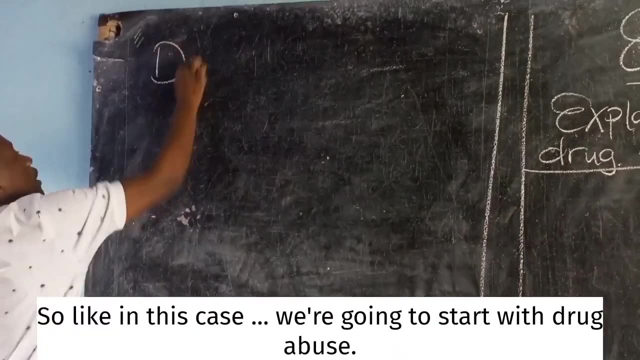 answering an essay question, start always by defining the key word. Like in this case, the key word is drug abuse. that's when you would link the opportunities that would be relevant- Yeah, that these could possibly be the causes. So, like in this case, we're going to start with drug abuse. 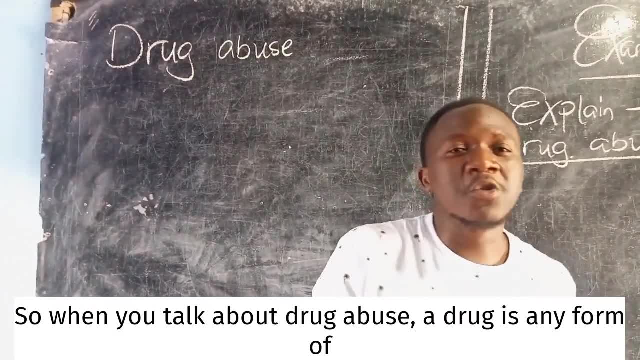 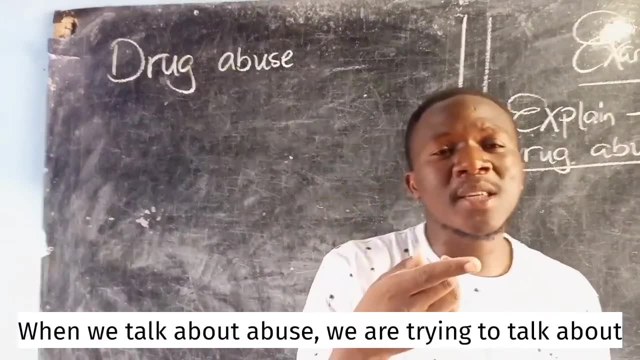 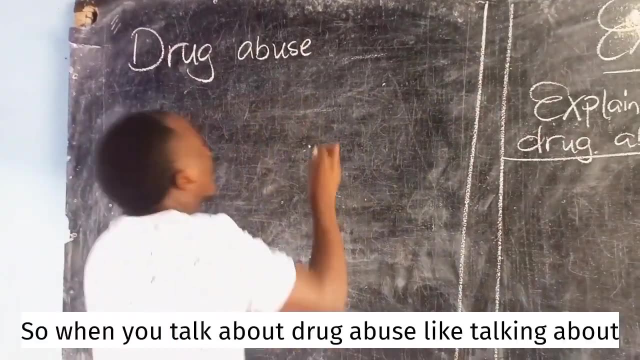 So when we talk about drug abuse, a drug is any form of material or any form of matter that can be taken in. When we talk about abuse, we are trying to talk about the misuse of something or the use of something for a wrong reason. So when we talk about drug abuse, we are talking about 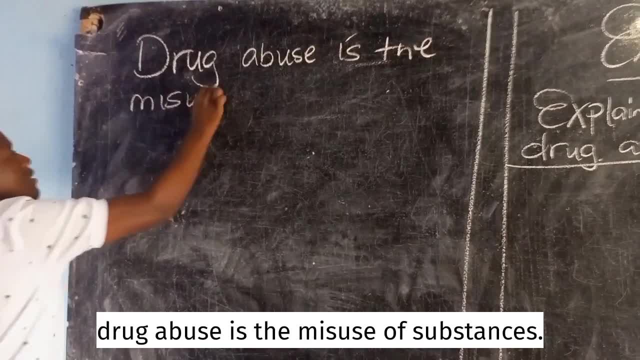 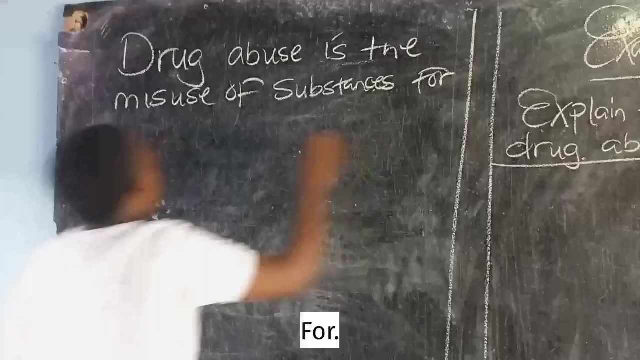 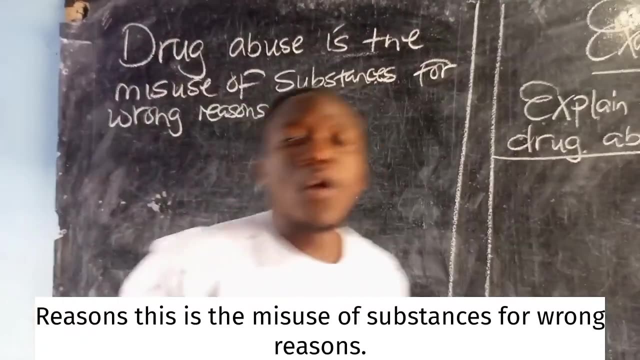 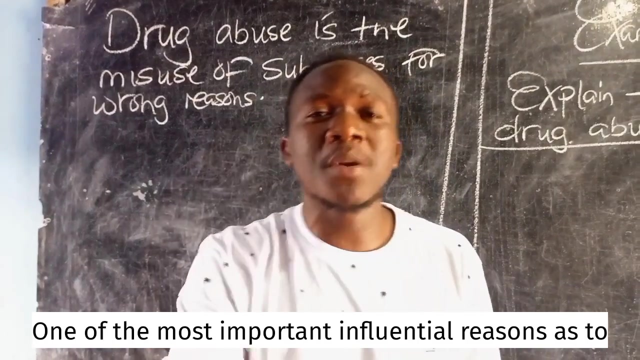 the drug abuse is the misuse of substances for wrong reasons. This is the misuse of substances for wrong reasons. One of the most important, influential reasons as to why lots of people do indulge in substance abuse, or drug abuse, is the misuse of substances for wrong reasons. 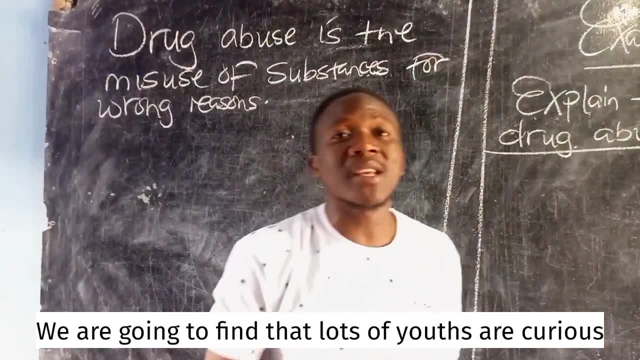 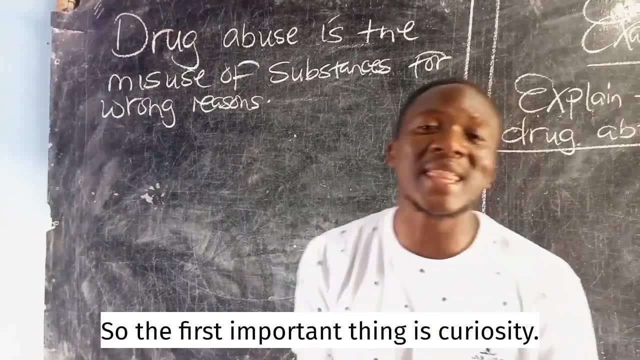 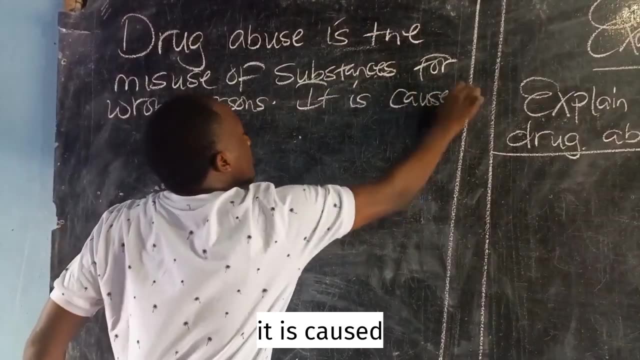 So when we talk about drug abuse, we're going to find that lots of youths are curious about knowing the effects or how well they would feel provided they took the substance. So the first important thing is curiosity. So we're going to find that it is caused by curiosity. It is caused 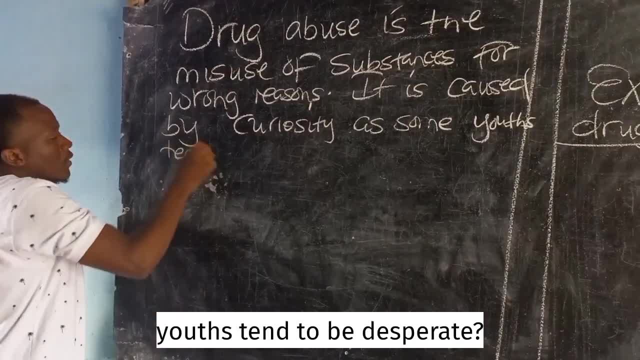 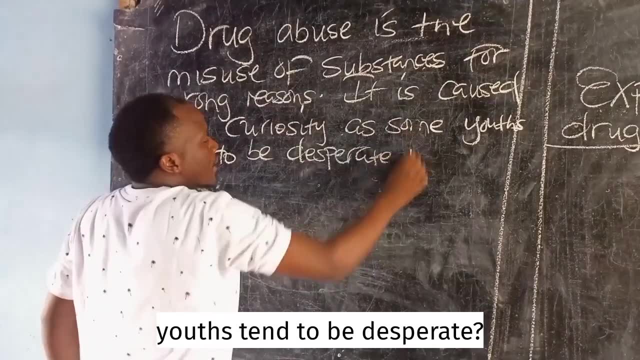 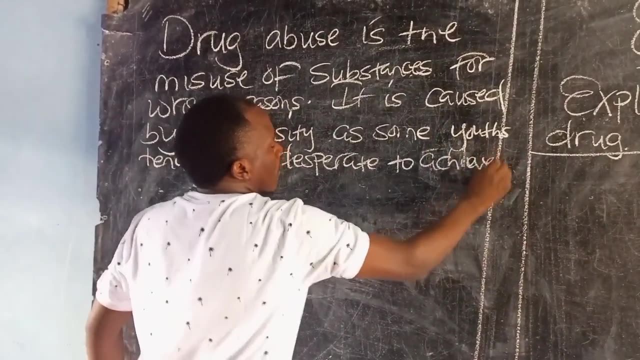 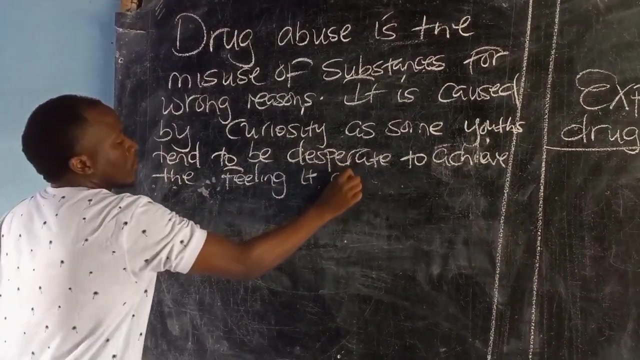 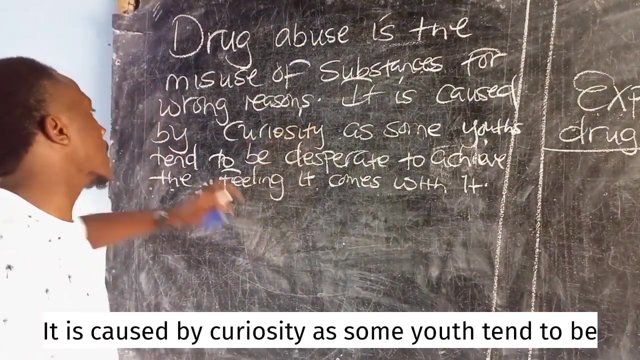 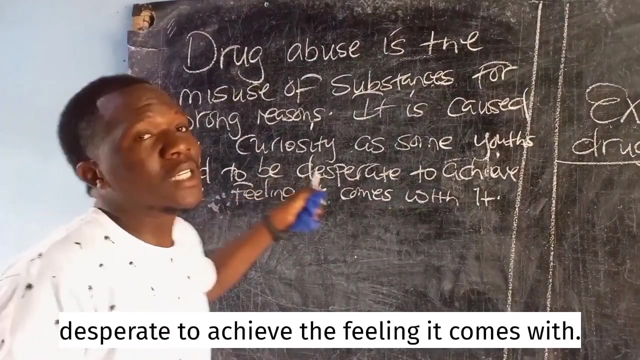 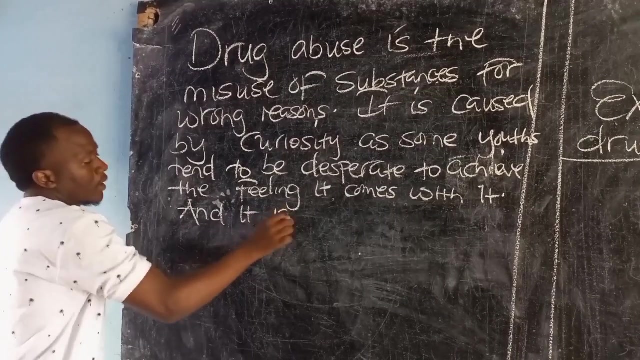 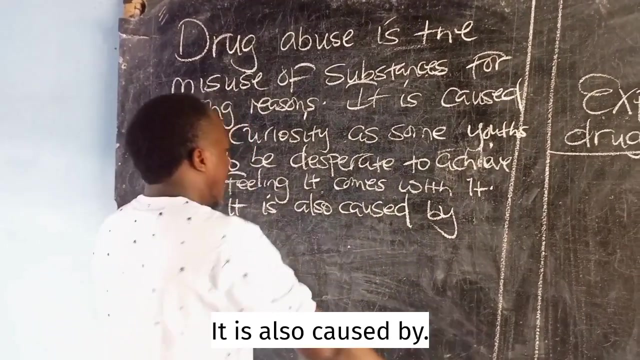 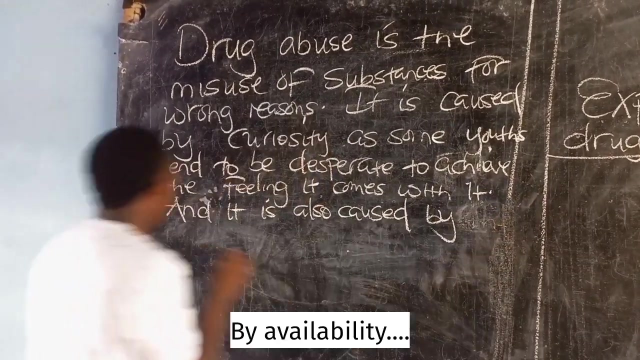 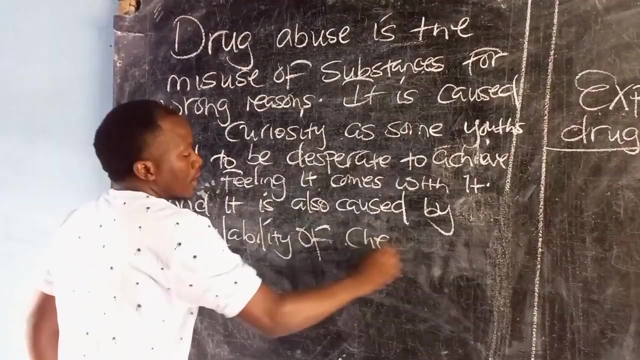 by some youths to be desperate. So this is our first point. It is caused by curiosity and some youths tend to be desperate to achieve the feeling it comes with it. Then, continually, we're going to say: and it is also caused by availability of cheap products. 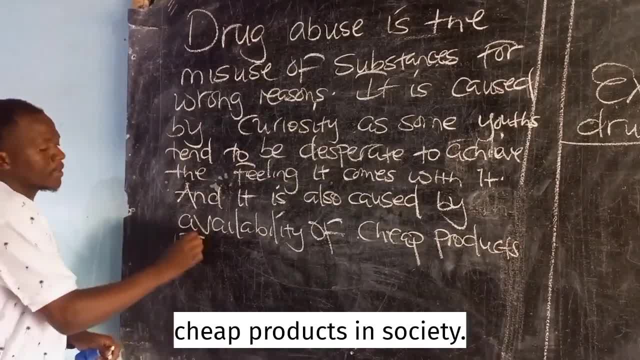 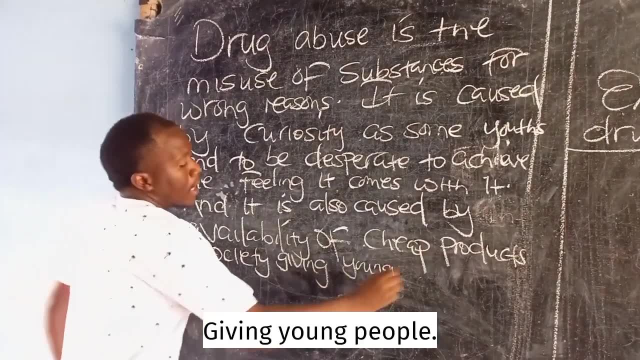 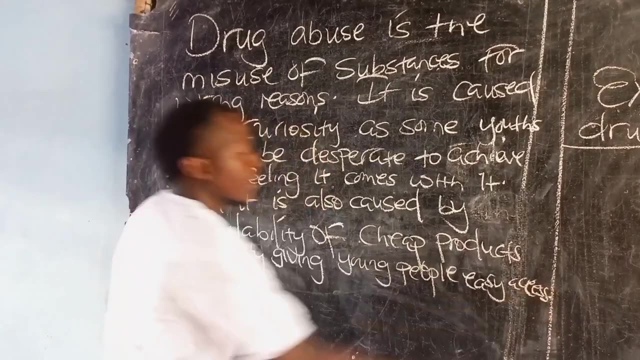 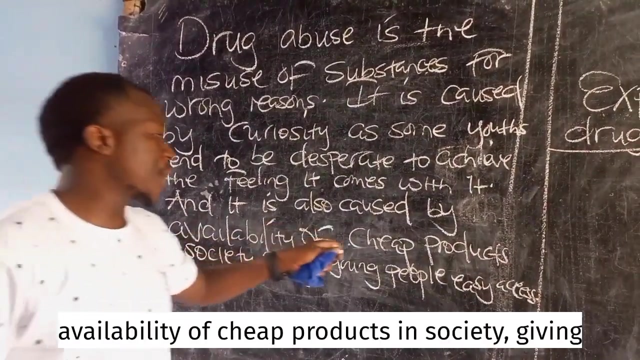 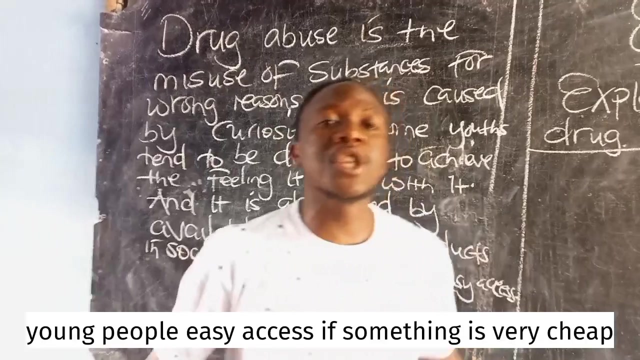 Availability of cheap products in society, giving young people easy access. So we can continue by saying: and it is also caused by availability of cheap products in society, giving young people easy access, If something is very cheap and then it is available, so that simply means the product is bought at a low price. 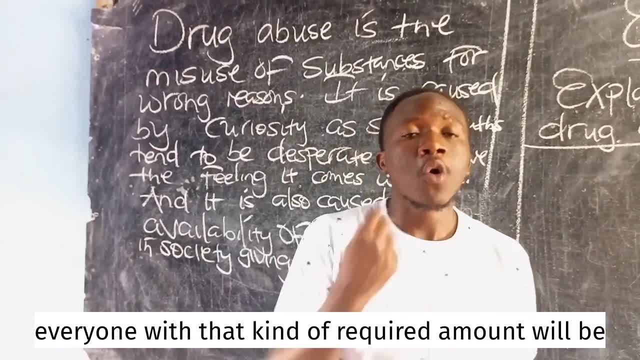 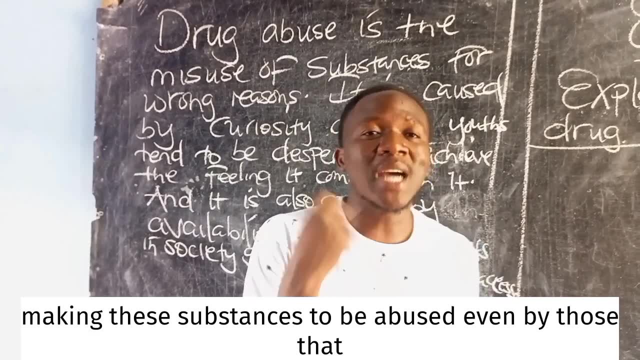 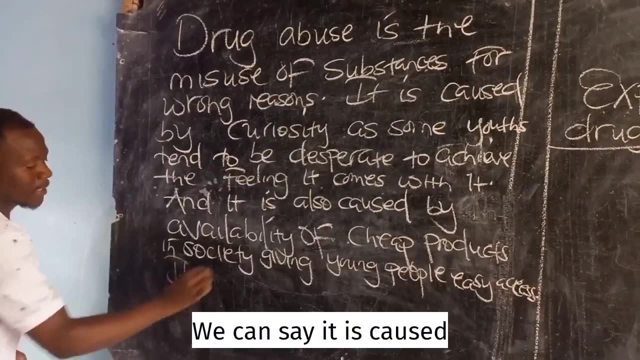 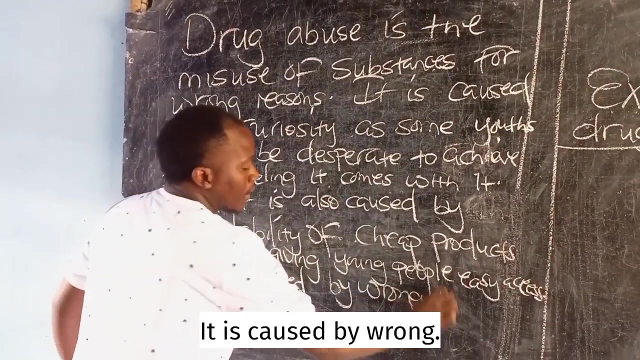 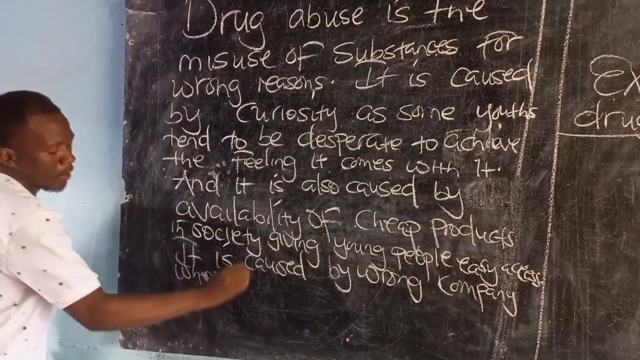 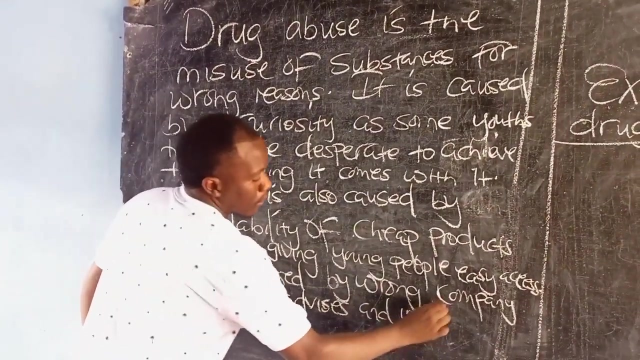 implying that everyone with that kind of required amount will be able to have access to the same product, thereby making these substances to be abused even by those that are minors or underage. Then, lastly, we can say it is caused. It is caused by wrong company, where bad advices and influence are offered. 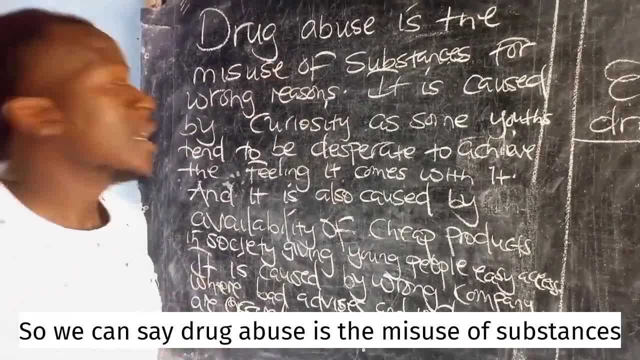 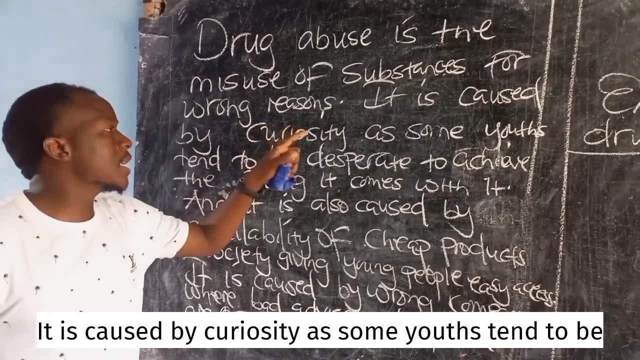 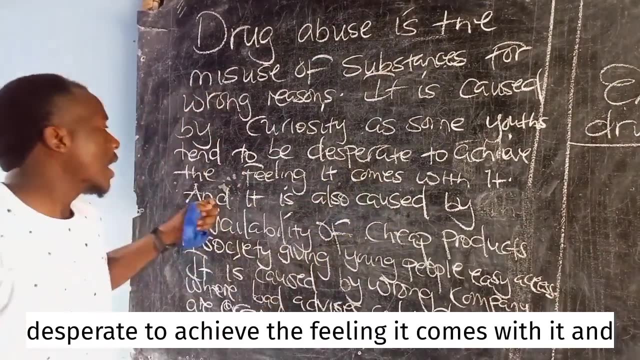 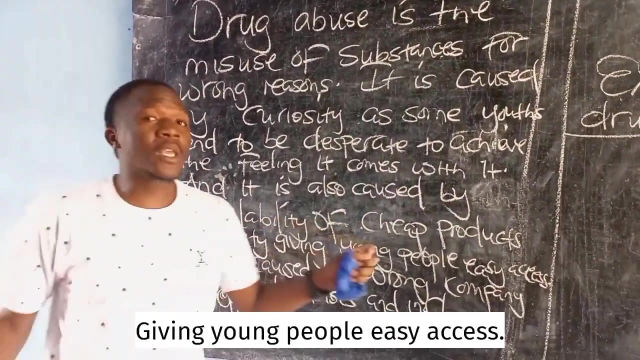 So we can say drug abuse is the misuse of substances for wrong. It is caused by curiosity and some youths tend to be desperate to achieve the feeling it comes with it, And it is caused by availability of cheap products in society, giving young people easy access.